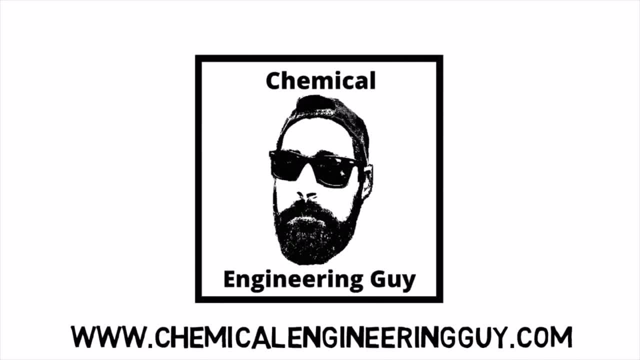 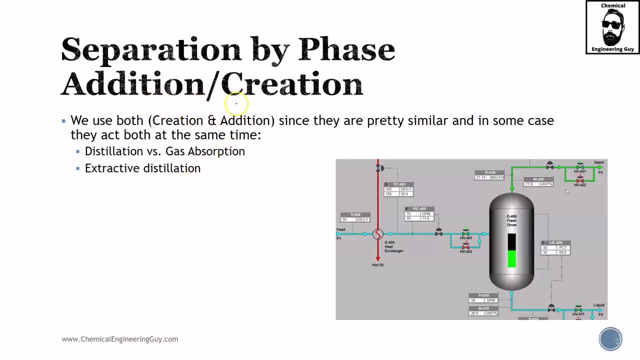 So I decided to include separation by phase addition and creation in the same section, instead of actually doing one separation for phase addition and another separation or another section for separation by phase creation. And I did this because I think this is pretty similar and you will encounter this a lot, and the processes don't vary that much between each. 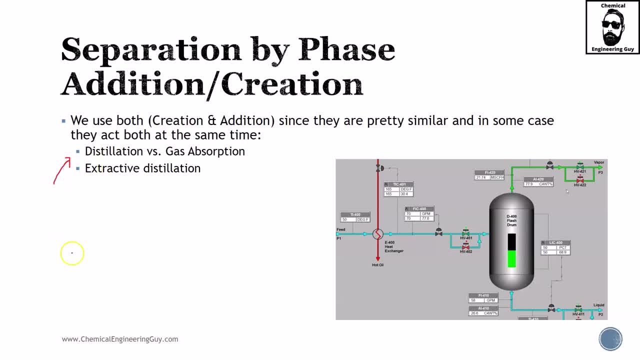 other. For instance, we have this special case, distillation, which we know. we have either a liquid or a vapor that goes inside and you separate a distillate, which is in vapor phase, and a liquid. So here you are creating one phase. If this was a liquid feed, then you are creating. 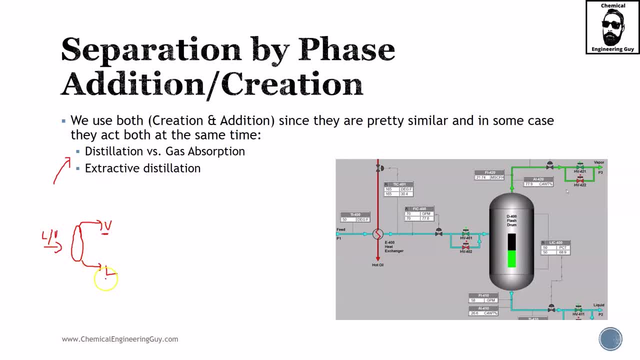 vapor feed and if you have vapor, you are creating a liquid feed For gas absorption. it's also, let's say, interesting that we are adding another phase. So we have our gas, which requires cleaning, so we add a liquid. So in these two cases it's very easy to separate them Actually. 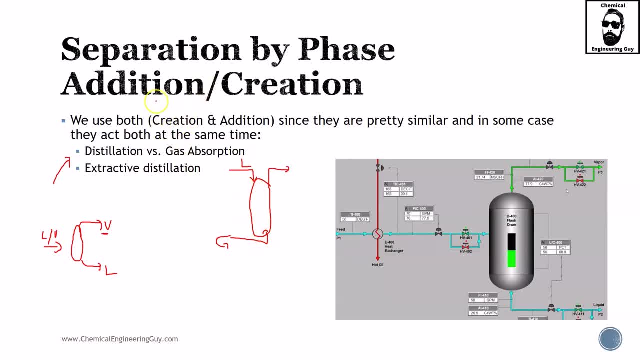 if I have to make a section for separation by phase addition and another one for phase creation, these two concepts or these two processes will be very easily separated. But what will happen then with extractive distillation or azeotropic distillation, In which we are going to see that we are adding another solvent? So let's say that this was a 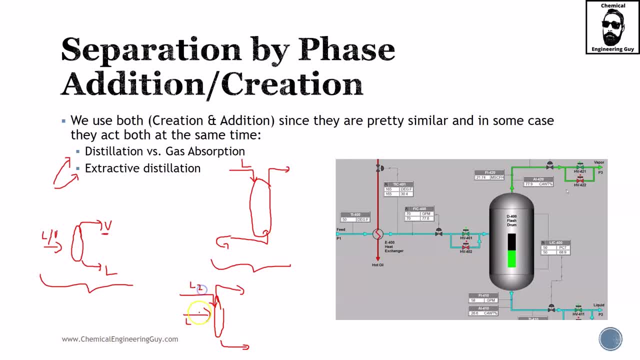 liquid phase and we are adding a second material in order to separate a vapor phase and another liquid right here Which later on is going to be separated into liquid one and liquid two. So what you will see in extractive distillation is that we have both phenomena, We have addition and creation. 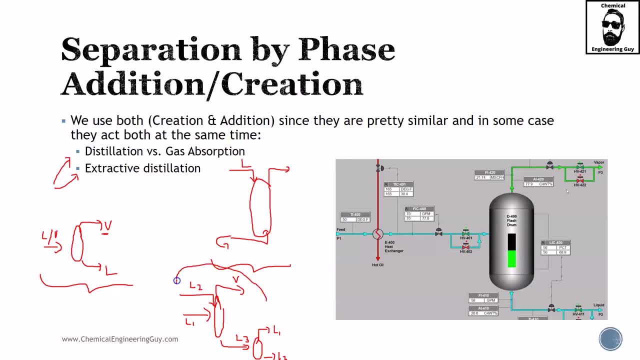 of phases. Now the main question will be: how are we going to categorize this process? Should we make this and arrange it in the same section as normal distillation, or should we add it to the second one? But, by definition, we are creating a phase, so that's why, in my opinion, it's much easier to 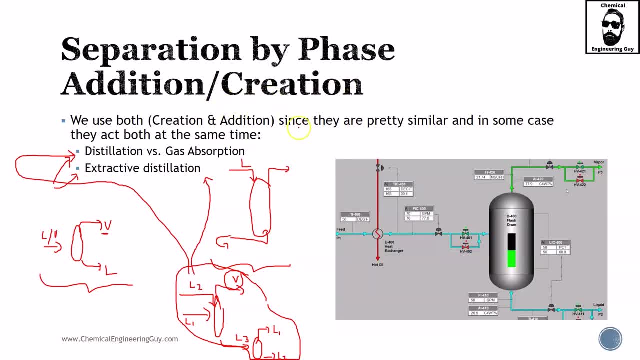 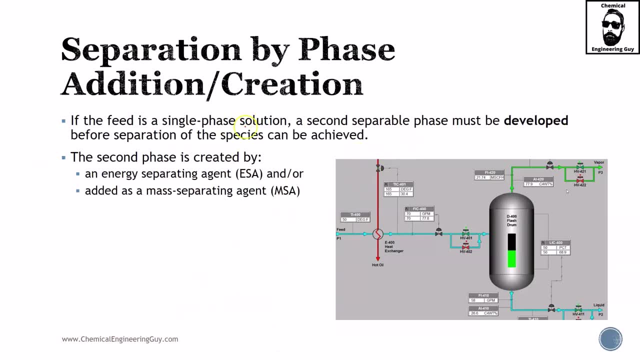 just assume that phase addition and phase creation are both pretty similar, and you will see that this is actually the case And it is much more convenient to analyze it this way. Okay, if the feed is a single phase solution, a second separable phase must be developed, So you: 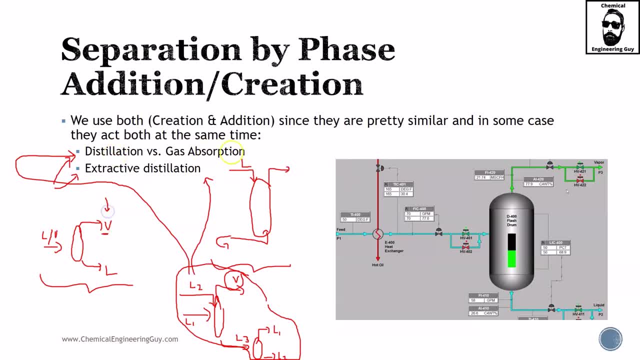 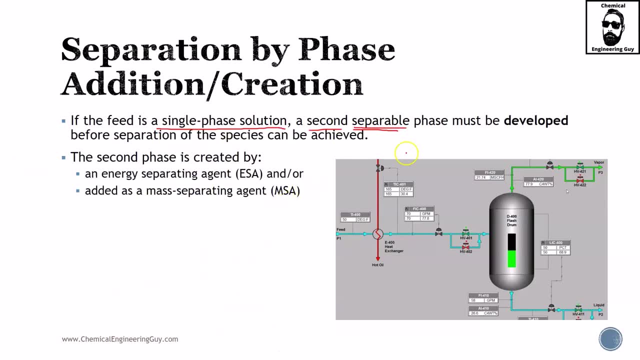 can see here, guys: in distillation you need to create a vapor. In gas absorption, you need to add a liquid. In extractive distillation, you need to add an entertainer. So, as you can see, a second phase, which is and must be separable, must be developed. So this is the main scope. 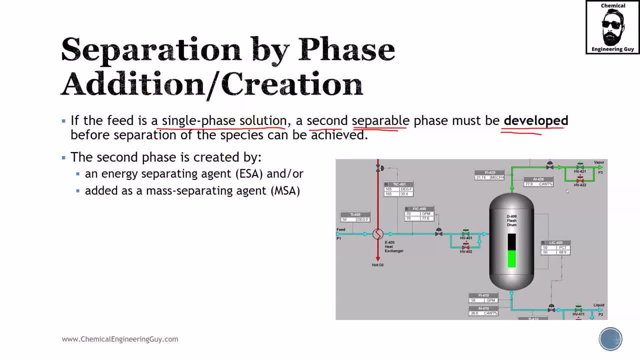 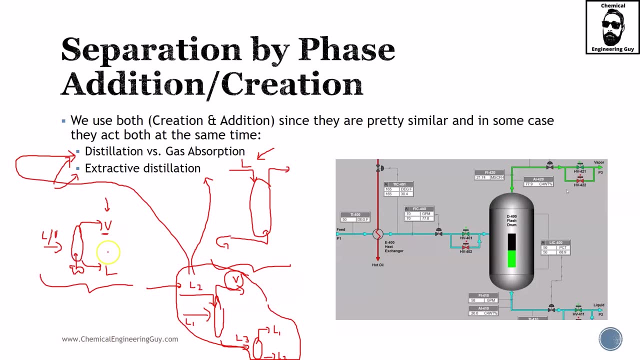 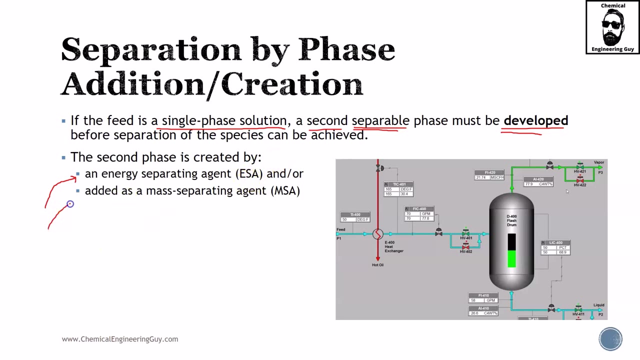 Okay, in the first phase, almost now the second phase- will be either created by energy separating Agent, ESA. So, for instance, in the distillation example you have a Reboiler which produces the vapor. that will be the, let's say that here heat is the technically speaking the ESA, but in the case of gas absorption you will be adding a. 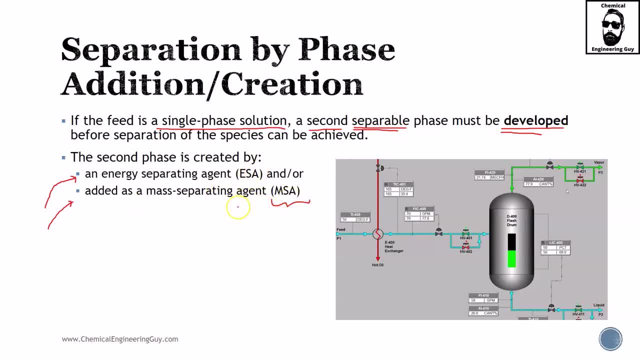 liquid, which is a mature mode of distillation, for example. how do we respond? how do we solidify this air and why the? so that's why we call this the MSA. So gas absorption is, by definition, MSA or requires MSA, and distillation requires, by definition, ESA. Now, as you can imagine you will for extractive. 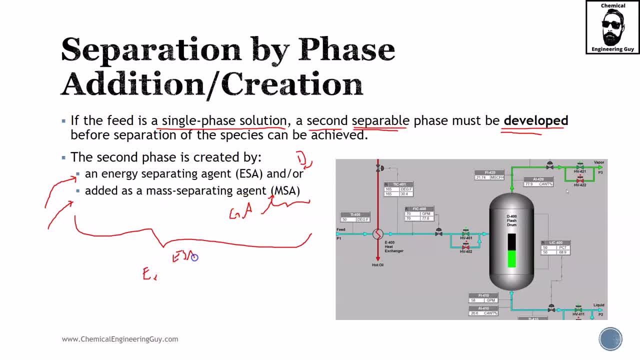 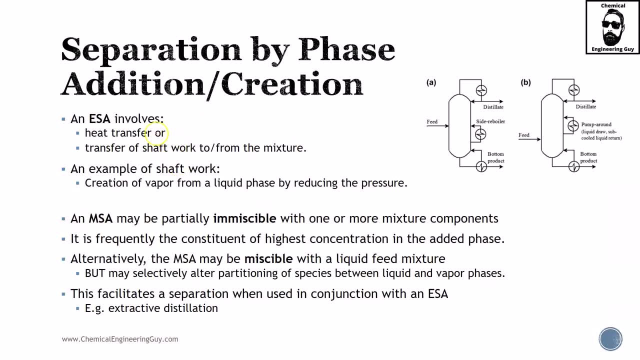 distillation. you will need both an ESA for the vapor creation and an MSA for the solvent addition. An ESA involves the heat transfer or transfer of shaft work we're going to see later on. You can use work in order to reduce pressure or increase pressure, not only heat. An example of shaft work: 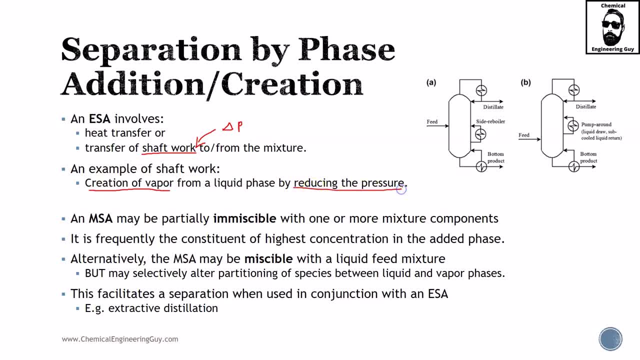 will be the creation of vapor due to the reduce in pressure in the system. So let's say that you have this flash drum and say that we have a piston right here and we remove it. What you're doing is increasing the volume. therefore, the heat transfer will be reduced, So you can see that the heat 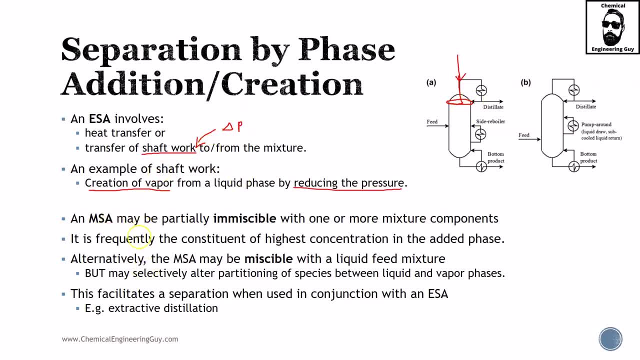 vapor must be created. An MSA may be partially immiscible with one or more mixtures, components, or must be separable in a certain manner, for instance in distillation. It is frequently the constituent of highest concentration in the added phase. so, going back in the extractive distillation, the entertainer 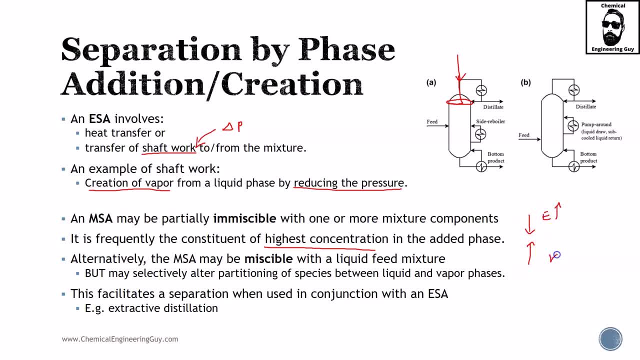 will be much higher than the actual- let's say, liquid or vapor- that we are going to separate. Alternatively, the MSA may be miscible with a liquid feed mixture, but in this specific case, as I told you, you will need to eventually. 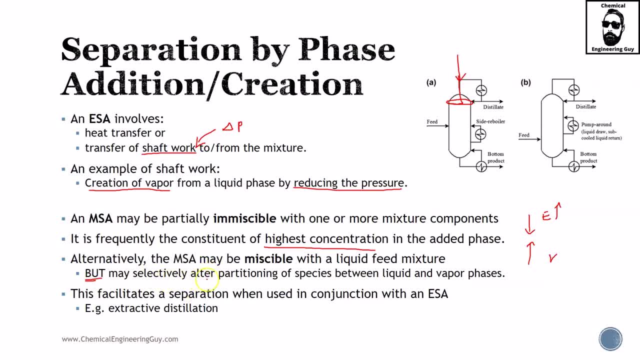 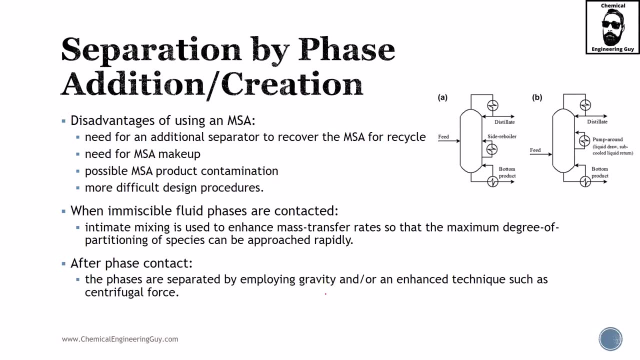 separate it, in this case maybe selectively alter partitioning species between the liquid and the vapor phase. This facilitates a separation such as in extractive distillation. Now, one of the main disadvantages of using MSA is, of course, if you are adding an extra material, you will need to separate them. sometimes it's pretty easy to separate sometimes. 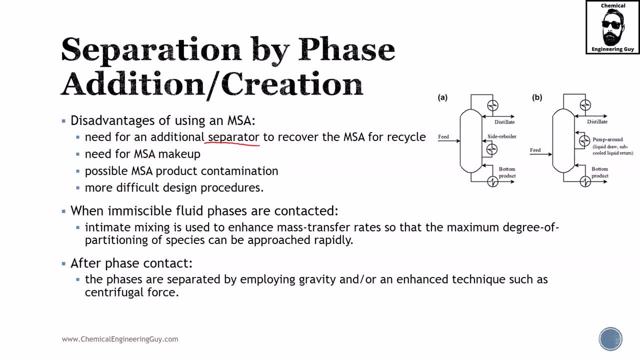 you will require a unique system for its separation and therefore you need a recycling, because if, once you separate these, you need to bring it back to the inlet, which implies a cost in pumping or in transport, You sometimes will be losing some material if you cannot separate these. 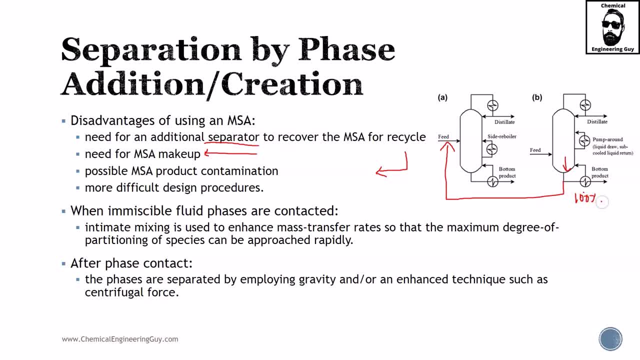 if not all the hundred percent of the MSA is coming here, let's say two percent is being lost in the product or in the vent. you will need to make up for that and also means that you need to spend some money on MSA. You can also come contaminate or pollute your material right. 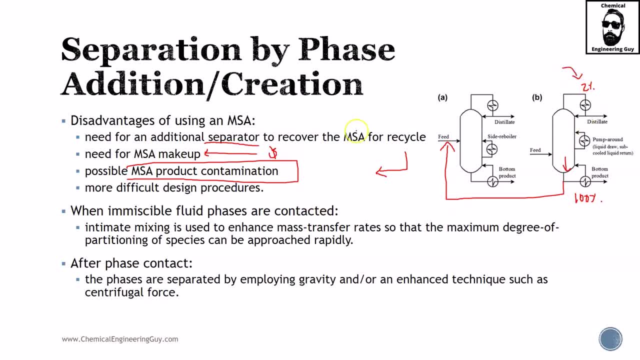 here this two percent. well then, this implies that you will need to decrease the quality of your final product, and so on. When immiscible fluid phases are contacted in the material, you will need to remove it and the quality of your final product will decrease. 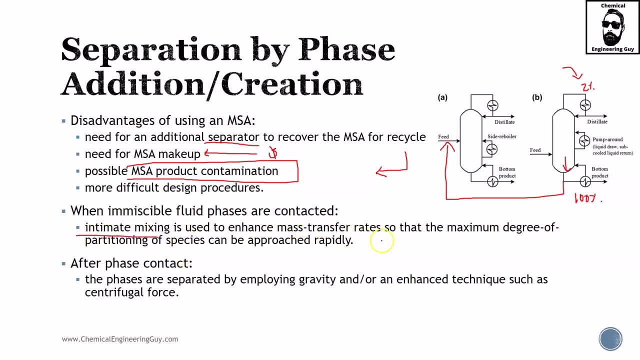 mixing is used to enhance the mass transfer rates so that the maximum degree of partitioning of species can be approached rapidly After phase contact. the phases are separated by employing gravity and or an enhanced technique such as centrifugal force. So once again, we are just repeating methods in which we can separate the MSA. For instance, here we're using 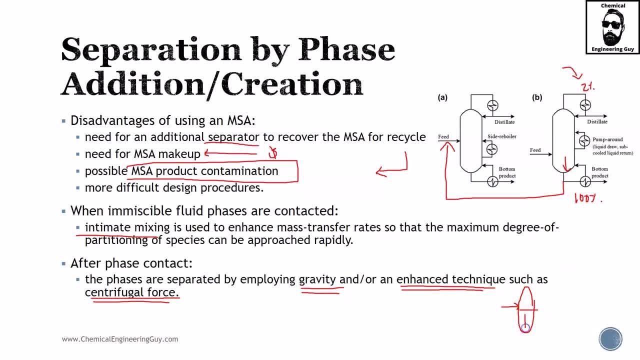 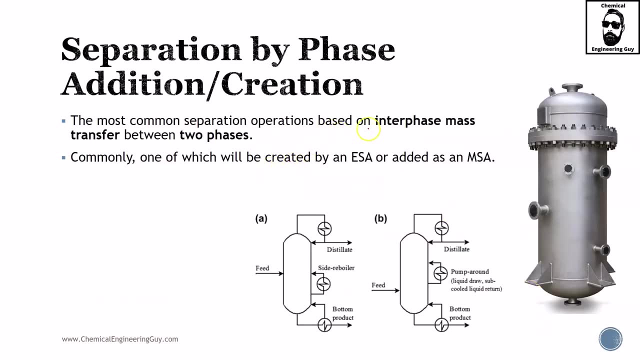 distillation, but easily you could use a decanter which separates, let's say, water and oil phase, and let's say that the oil phase is here, which is our product, and let's say the aqueous phase contains our MSA, well then, you will be able to remove it, The most common separation operation.